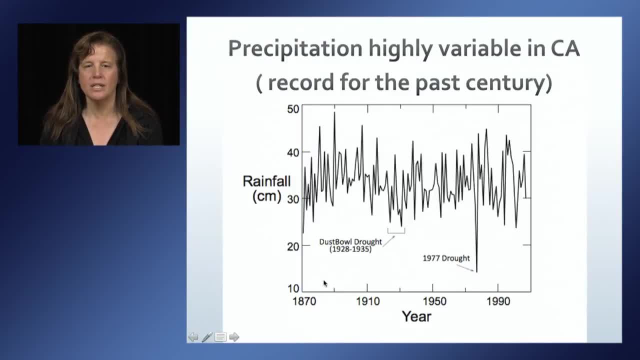 So if we look at this graph of precipitation from 1870 to about 2000,- we have, for example, rainfall on the vertical axis in centimeters per year and time in years before present on the horizontal axis. You can see that precipitation is highly variable. Much of this variability. 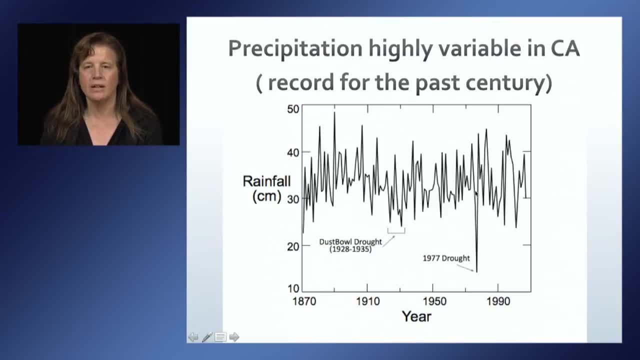 is due to El Niño and La Niña, so conditions over the Pacific Ocean that bring storms more or fewer, or greater in number of storms. So the case of the Pacific Ocean has been that it brings storms to California each year, And some notable dry years were the 1977 drought and the Dust Bowl drought in 1928 to 1935. 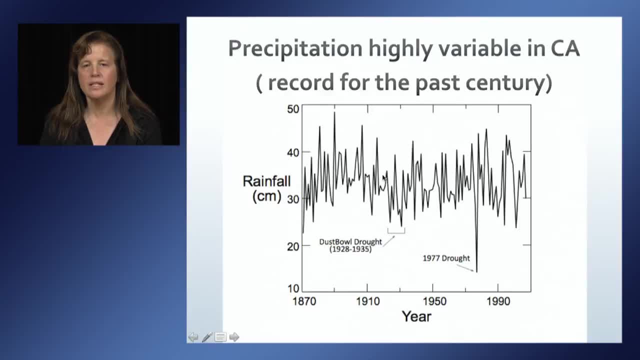 And you can also see that there's a longer-term average variability that is related to the Pacific Decadal Oscillation, so it's more a 20-30 year variability in precipitation. So if we look at the Pacific Ocean, we have the Pacific Ocean in the upper middle of the 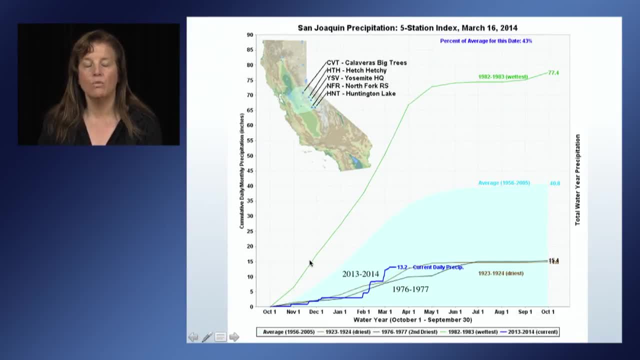 So if we look at the water year, which begins on October 1st and goes until September 30th, just to compare this year with those previous years, you can see in blue: this is 2013-2014, beginning October 1st and this is the cumulative precipitation. 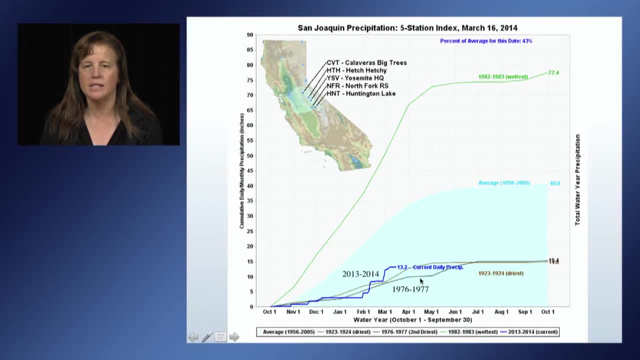 And if you see these other curves, this is 1976-1977.. So we're currently, as of March 16th. we're higher than 1976-1977 and 1923-1924.. So, depending what happens, the remainder of this water year will either be slightly below, 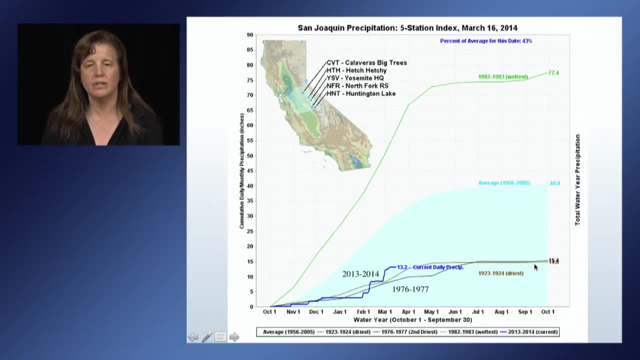 or perhaps on par with the two driest years on record, And this is a record for central California. This is a record for central California. This is a record for central California And this green is showing 1982-83, which was the wettest year on record. 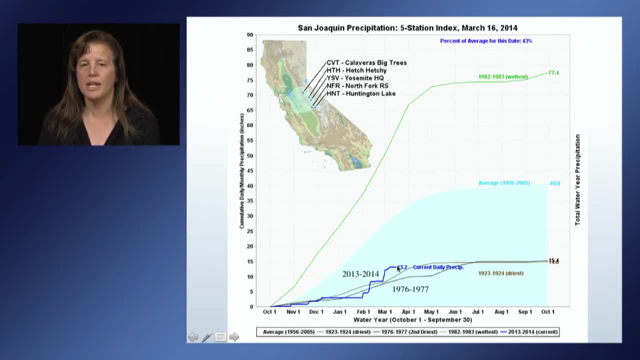 And we're currently about 40% to 50% of the average. So this blue is showing the average over the entire period. So another question is: well, how does this year compare to the last few hundred years? And for that we actually have to look back in the natural archives. 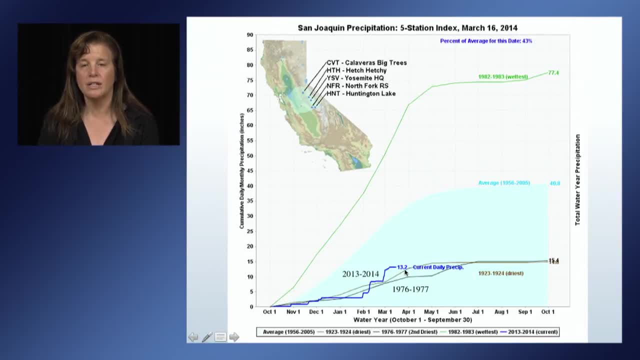 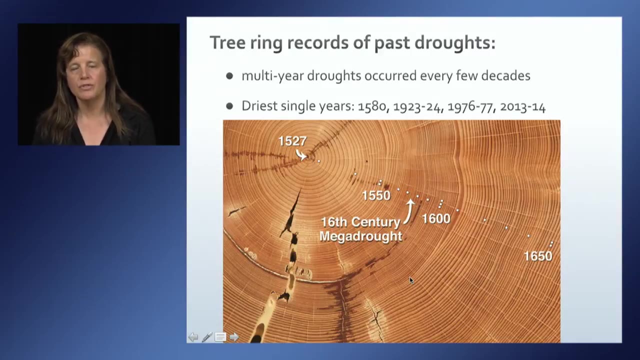 We don't have recorded history beyond the late 1800s, so we have to look into tree rings and sediment cores and things like that to really understand the longer-term history of water. And so if we look at this tree ring record for the past 500 years or so, what these tree? 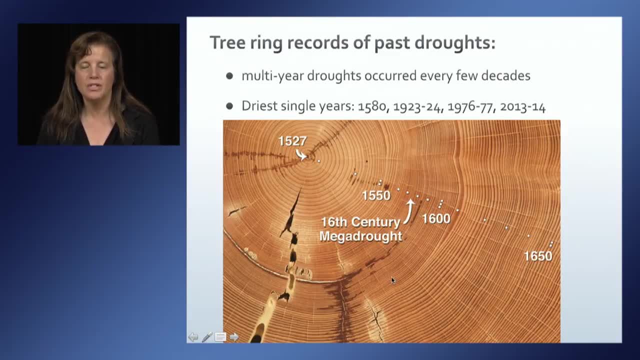 ring records show is that multi-year droughts occurred every few decades, and the single driest years occurred in 1580,, 1923-24,, 1976-77, and potentially this year, 2013-14,, if we. 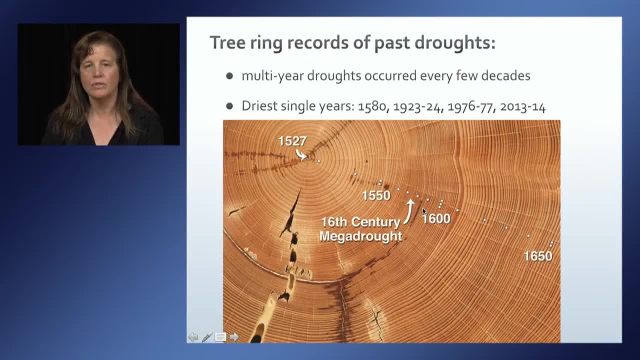 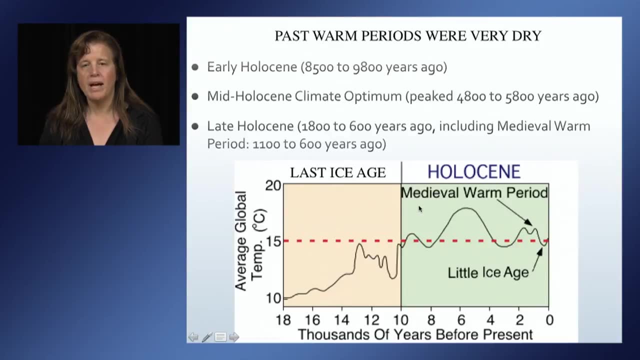 compare it with the long-term record, So we're within the four driest years of the past 500 years. If we look back over a much longer period of time, this is a record of climate. It's showing the average global temperature on the vertical axis, so it's 10 to 20 degrees. 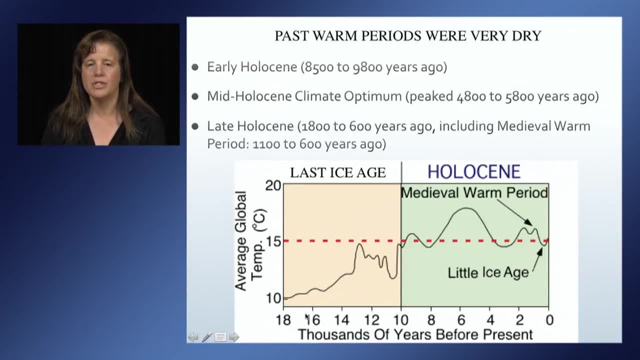 here Celsius versus time, So this is thousands of years ago. So here we are at the present, at zero going back in time. here's 2,000, 4,000 years heading back in time, And the beige color here is representing the last ice age. and then we transition into: 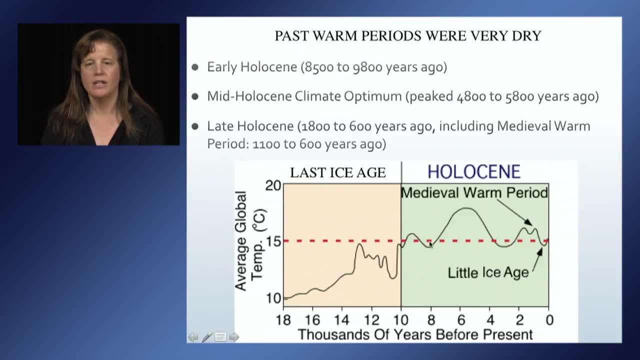 our current warmer holocene, And so you can see that there were three generally warm time periods within our current warm period. We have the early holocene period from 8,500 to 9,800 years ago. that was also dry. Then we have the mid-holocene climate optimum that peaked 4,800 to 5,800 years ago and 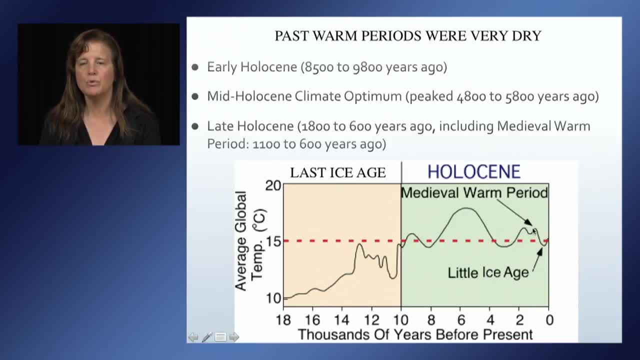 again that was a very dry period. So we have the mid-holocene climate optimum that peaked 4,800 to 5,800 years ago and again that was a very dry period. And then, if we move forward to the medieval warm period in the late holocene generally, 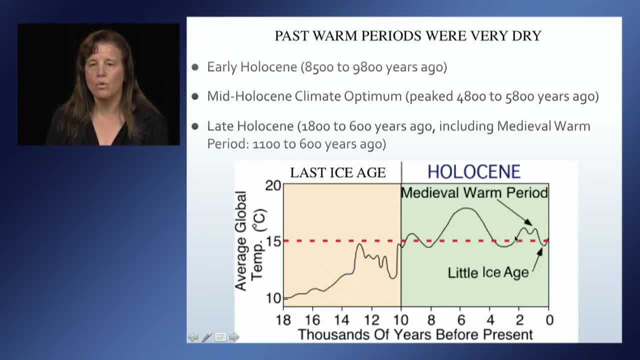 from 1,800 to 600 years ago it was warmer and again it was drier, And it was particularly dry during the medieval warm period 1,100 to 600 years ago. So I'm going to focus on right now, on the evidence for why it was drier during that. 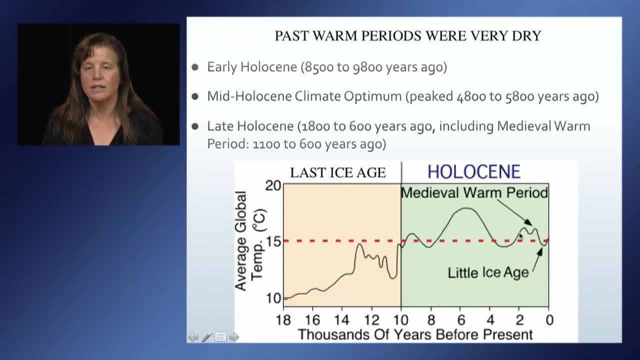 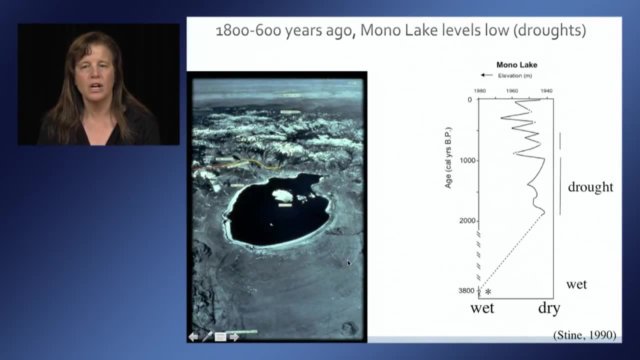 time, in fact, with droughts lasting over a century. So some of the first evidence we had was from Mono Lake- and this is the work of Professor Scott Stein at Cal State, East Bay- And he looked at the lake level or the size of this lake. 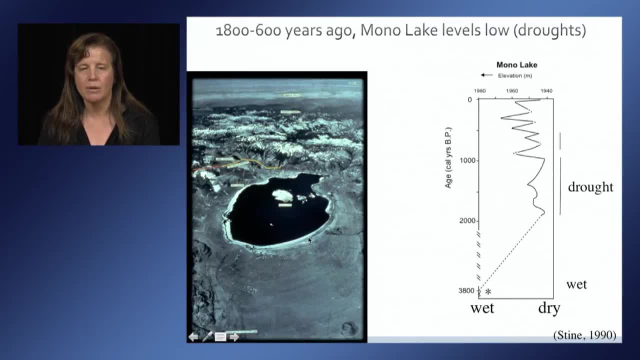 The lake expands during wetter times, During drier times, the lake contracts, And this lake is in the eastern California, east of Yosemite Park, And so what is plotted here is age, With the present at the top. going back in time, here's 1,000 years ago, 2,000 years. 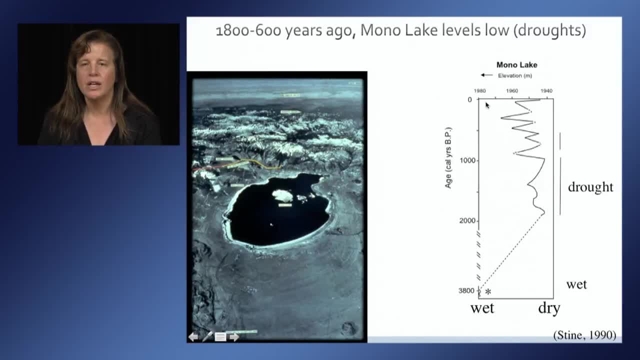 ago And that's plotted against the lake level, And so higher lake levels are to the left, lower lake levels to the right, So it was drier when the lake level was over here to the right. So what you can see is that there's this extended period where the lake was low, it was dry. 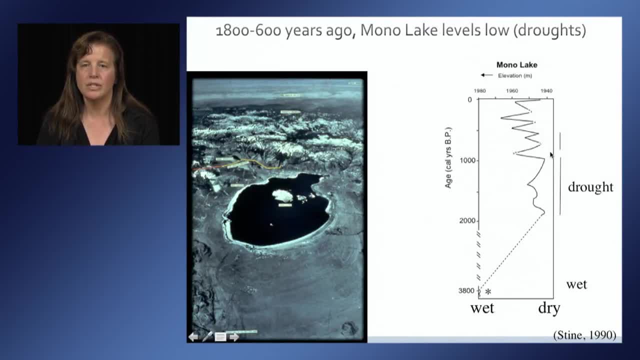 between 1,800 and 600 years ago, And you can also see that over the last 1,000 years or so there's been some fluctuations- wet-dry, with a period of about 200 years. So every 200 years it got wet and then dry, again, wet-dry. 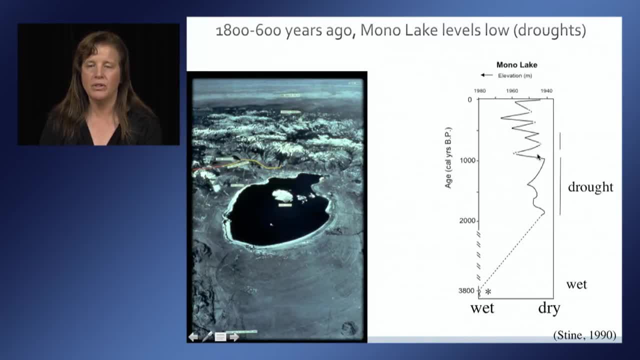 So I'm going to now talk about this medieval period here, between 900 and 1,400 AD. So when you have a period of about 200 years, it's a later period. We'll talk about that later. There was a period between 900 and 1,400 AD. 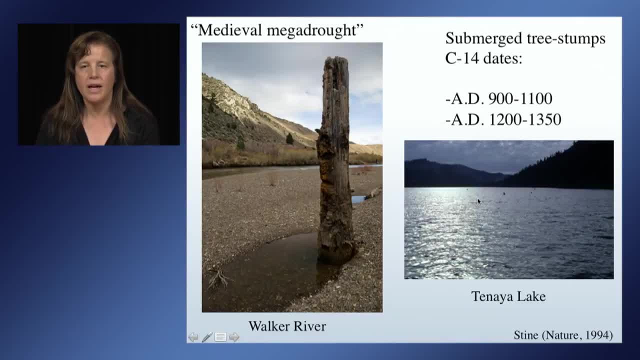 Between 1,400 and 1,400 AD. So this is an example here. So this is a very nice map. So this is an example here, So this is a very nice map And this is evidence that again, Scott Stein discovered. 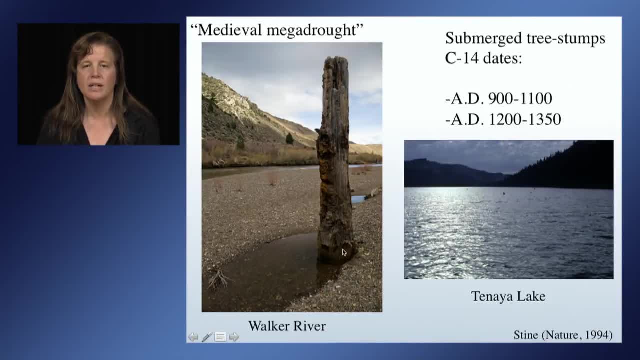 which was these submerged tree stumps. So throughout the Sierra Nevada he noticed that in places that are now bodies of water or rivers, there were tree stumps that are rooted in these bodies of water that suggest that sometime in the past that that body of water had dried up. 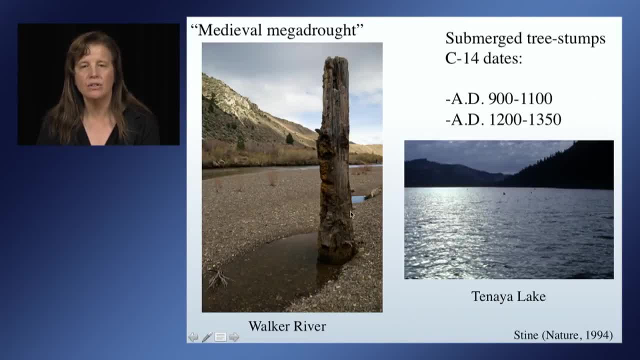 or that river had dried up. So he actually radiocarbon dated the outer rings of these trees to get the age that the trees died, And what he noticed was that these trees that the radiocarbon dates came out into two generations of stumps. 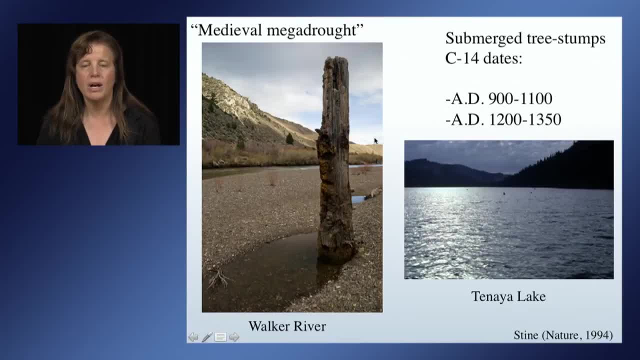 meaning two droughts, And so by actually counting the tree rings, he could get the age of the trees, how long the trees had actually grown there, And he found out that there were two droughts, one between 900 and 1100 AD. 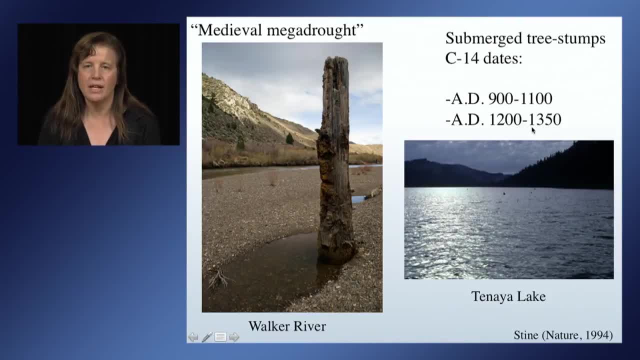 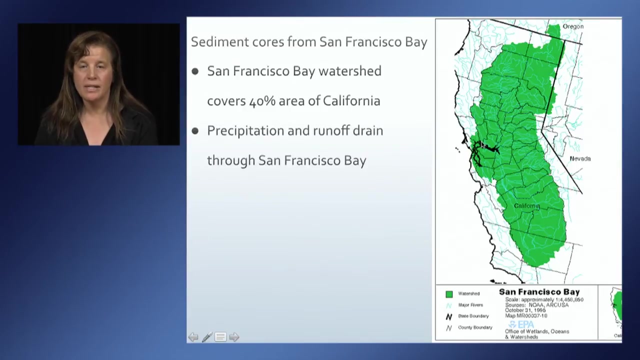 and the next one from 1200 to 1350 AD, And so these are called the medieval mega-droughts. They're these very extended periods of dry, perhaps 60% of average precipitation that occurred during that medieval time, And so in my laboratory we work on sediment cores. 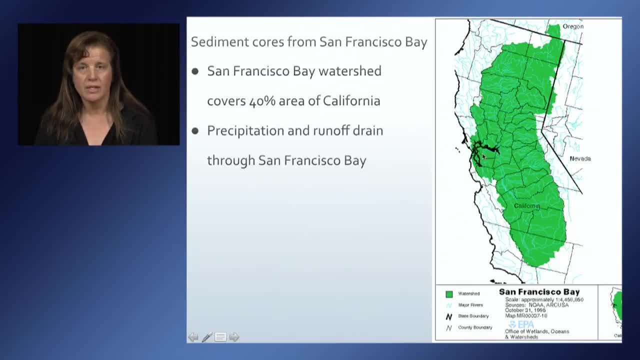 And so we. one of our ongoing projects has been sediment cores from San Francisco Bay, and the reason that we're looking in San Francisco Bay is that its watershed covers 40% of California, so you can see this green area. here is the watershed for California, for San Francisco Bay. that, so all of the precipitation and 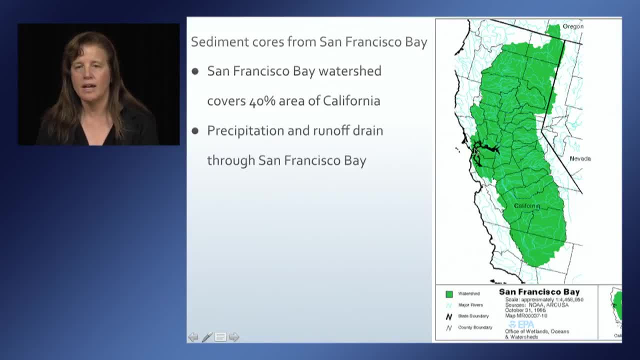 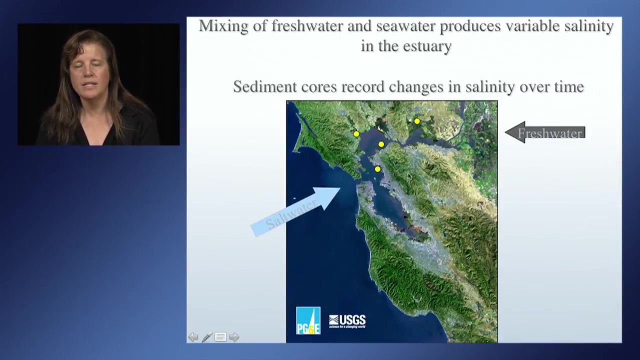 runoff over this area, drains through the Delta and into San Francisco Bay and then out into the Pacific Ocean, and so if you look at the salinity in the Bay, you can. actually the salinity reflects precipitation and runoff from a very large area, California, and so our idea was that if we had a way of determining 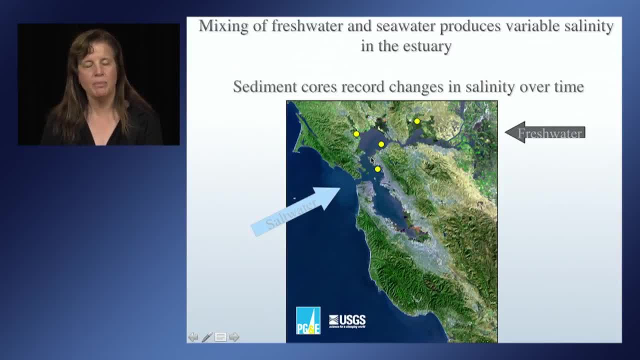 past salinity. we could then determine pass precipitation over a large area of California, because as fresh water comes into the bay, it mixes with salt water and you can actually. the salinity at various locations in the bay is directly controlled by the amount of fresh water coming into the estuary. 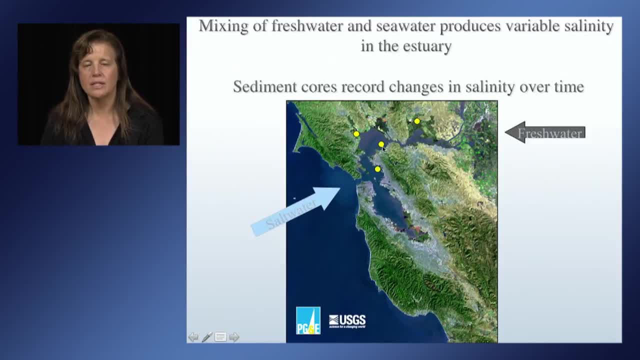 So we took sediment cores from various locations indicated by these yellow dots and looked at the chemistry of the sediments and the fossil composition of the sediments, And then we dated the cores with radiocarbon and that way we could get a record of past. 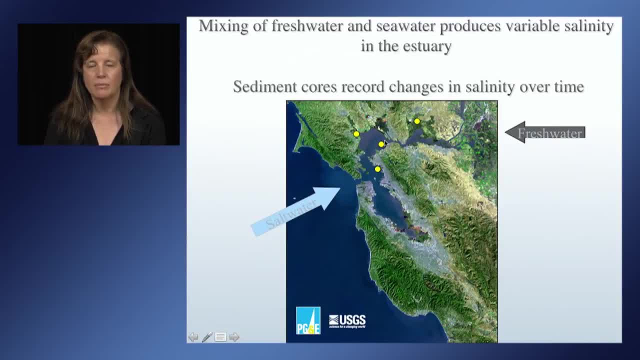 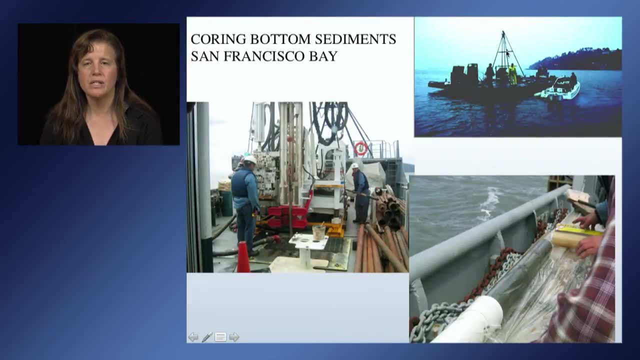 floods and droughts or wet and dry periods over the bay's watershed, And so over the years we've gone out with various types of drilling platforms. This was a drill ship And this is showing what they look like, What the core looks like. 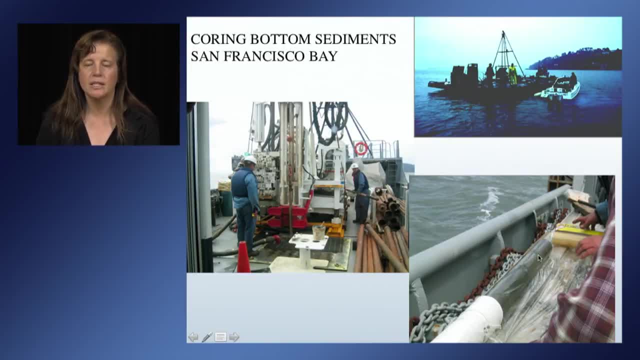 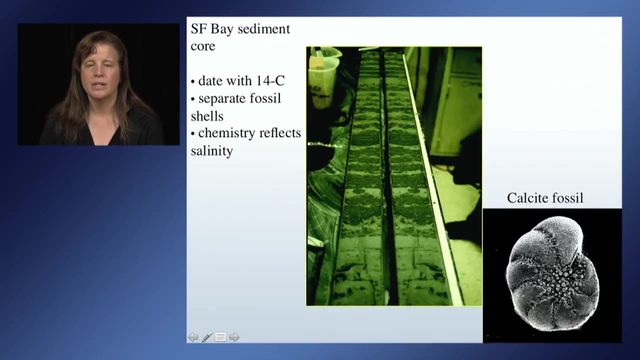 It's several, maybe three inch diameter and generally just clay sediment, fine grained silt and clay- but also contains lots of fossils that we can use to look at past salinity. So this is an image of the core split in half and you can see this general layering of the 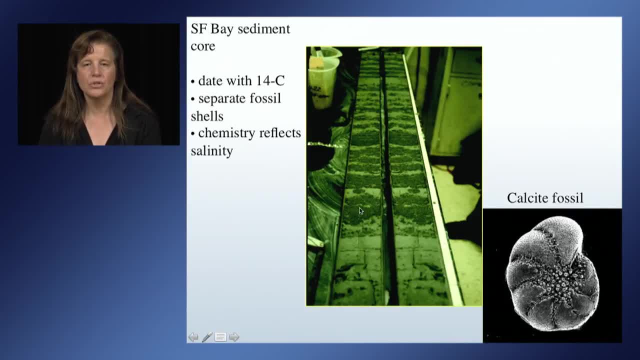 core, And this is a picture of the core with finer grain sediments and coarser grain sands. And so we first dated this core using radiocarbon methods and then separated out fossil shells from the cores, And we looked at both the type of fossils, because different organisms live in different 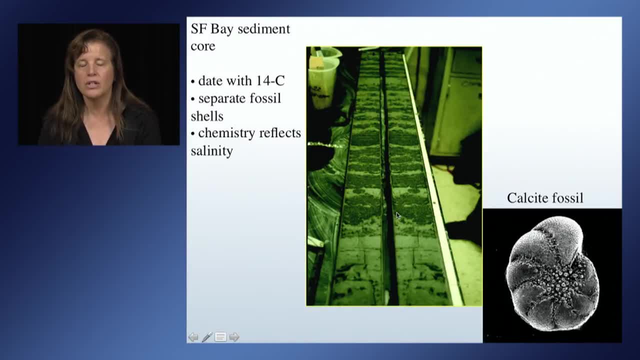 conditions of water. So some prefer saltier water, some fresher water. So that was one measure of the salinity. But then we also could look at different organisms living in different conditions of water. So we looked at the chemistry of the shells that reflect salinity. 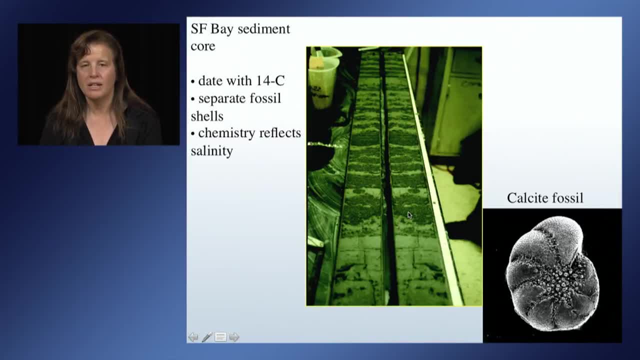 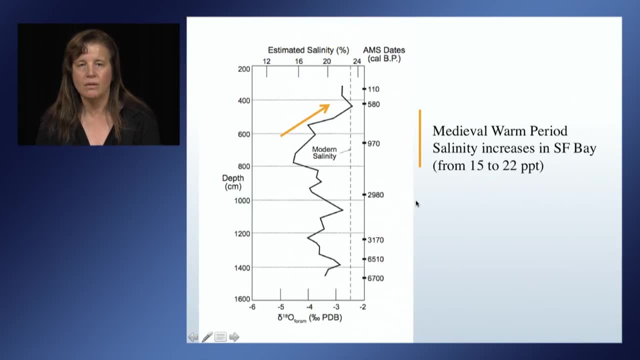 And I don't have time today to explain those exact methods, but it's using isotopes of oxygen, So this is the record that we came up with then. So on the top, here is the estimated salinity, And so here's 12 to 24 parts per thousand. 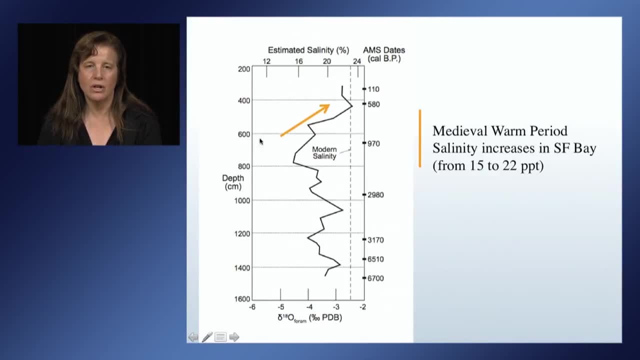 So here's the estimated salinity. So here's 12 to 24 parts per thousand. So we've got this depth in the core on the vertical axis, And then I've also added the radiocarbon ages here. So what you can see is that there was this. well, we see these shifts in salinity reflecting. 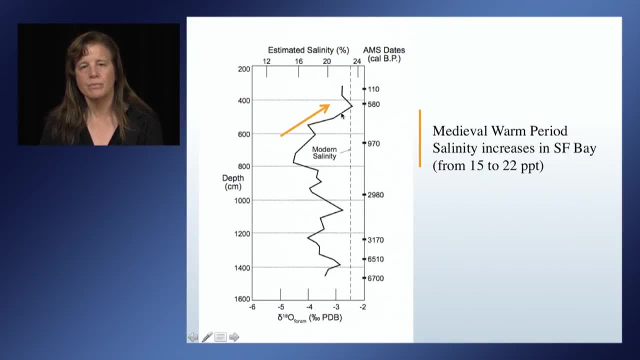 wet and dry conditions. But then there's this very significant increase in salinity that occurred during that medieval warm period where we saw elsewhere in California that there was There were drier conditions. We see that in the estuary salinity increased from 15 to 22 parts per thousand over this. 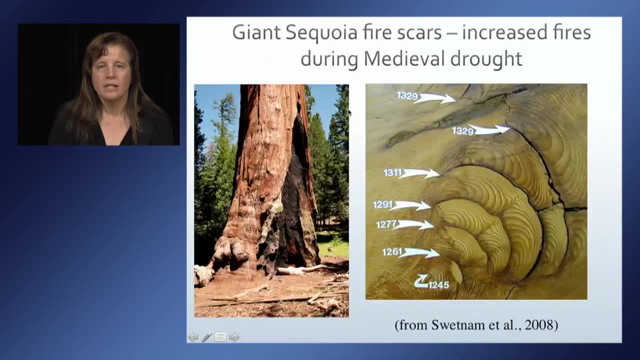 dry period. If we go back to the Sierras now and look at giant sequoias, this is the work of Thomas Swetnam at the Tree Ring Lab at University of Arizona. What he is seeing You can. actually, These trees often do not can survive a fire and they actually form a fire scar during. 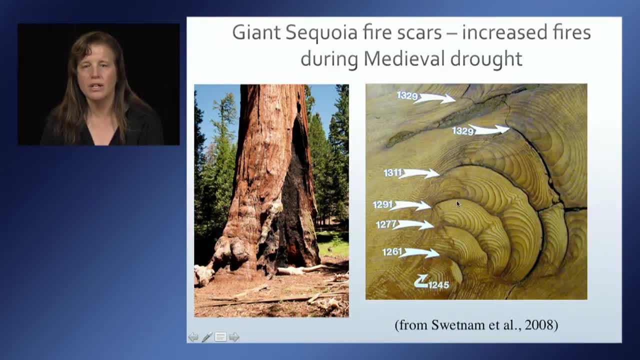 a fire And if you look at a cross section of the tree trunk, you can actually see these past fire scars and you can date them. And so he's shown with these numbers: 1311, 1277 and so on are the actual dates of these. 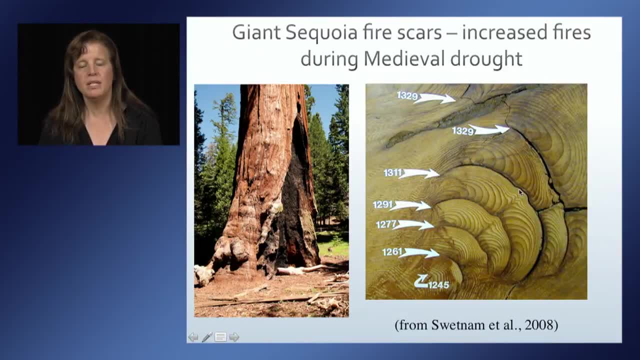 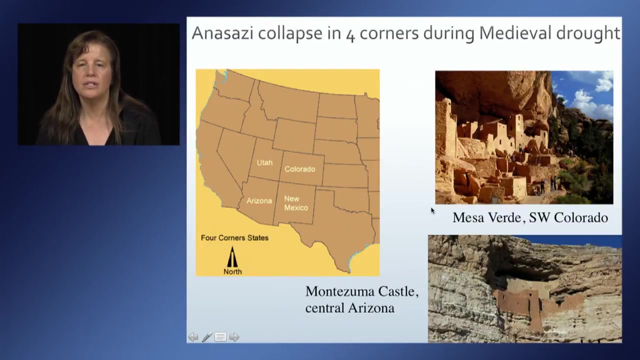 fires And what he was able to piece together using lots of trees And what he was able to do with these trees from Yosemite National Park, was that the fire frequency was much greater during that medieval dry period. It went up about 30% And the other effect that we see during 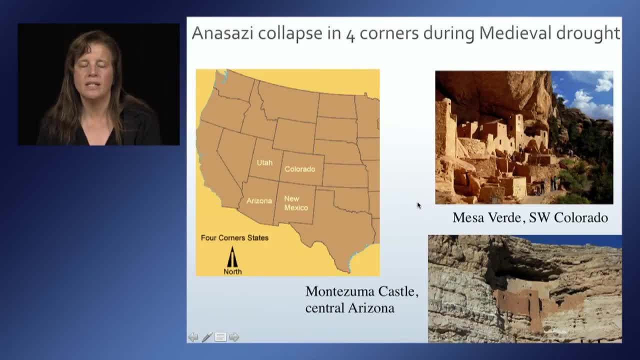 Toward. the end of that medieval dry period was the collapse of the civilizations that were living in the Four Corners region As well as along the coast in California. we have archeological deposits of shell mounds that appear to be abandoned as well at the end of that drought. 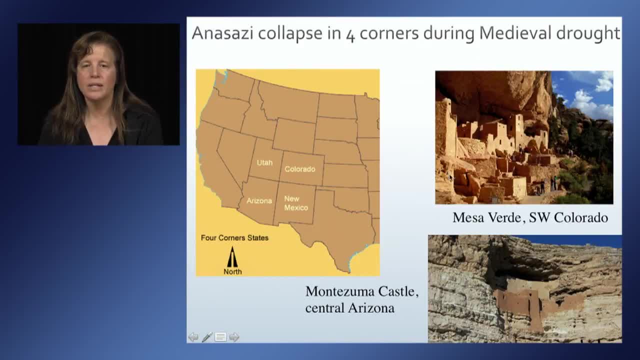 So this is showing Mesa Verde in Southwest Colorado and here's Montezuma Castle in Central Arizona. So the archeological evidence shows that there was starvation, malnutrition and even conflict and violence Between groups. as resources dried up and dwindled, you had competition increasing. 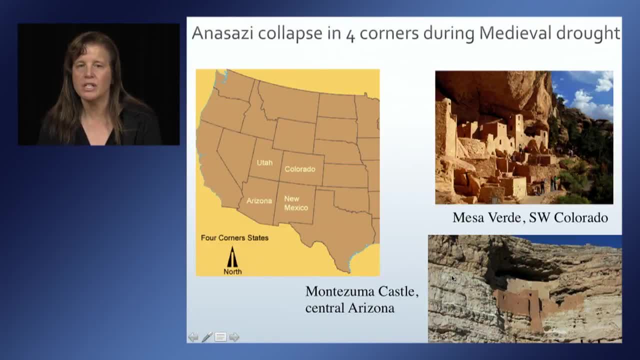 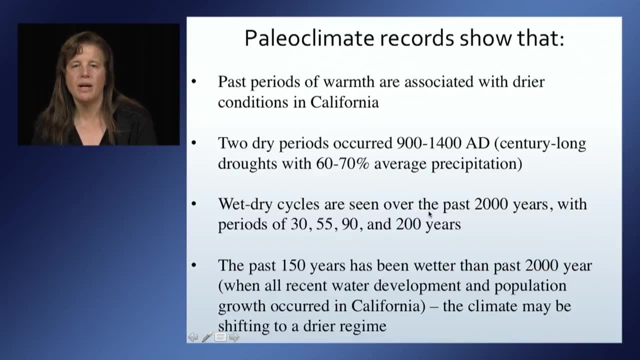 competition for those resources And, finally, mass migration in search of more water and resources. So, to sum up what we've talked about, the paleoclimate record shows that past periods of warmth are associated with drier conditions in California, And that's a good thing. 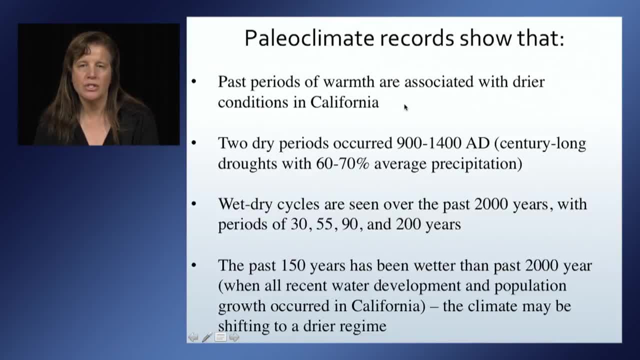 There were two periods, dry periods that occurred between 19 and 1400 AD during this medieval warm period. These were century-long droughts, two century-long droughts that had 60 to 70% average precipitation. We also see wet-dry cycles over the past 2,000 years, with periods of 30,, 55,, 90, and 200. 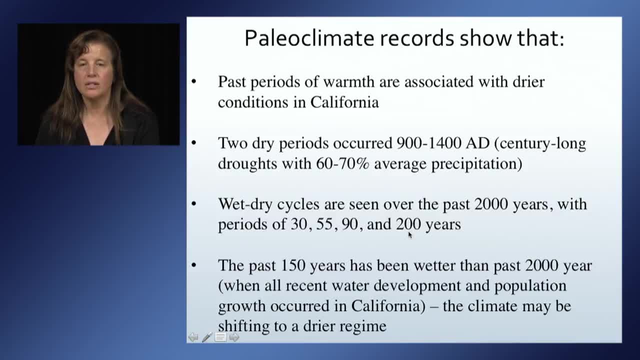 years, So there's other variability. It's a good thing, And we also note that the past 150 years have been unusually wet when viewed over the past 2,000 years. So the 20th century was a wetter century. 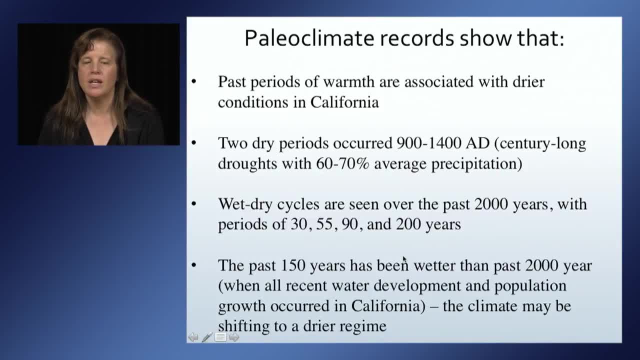 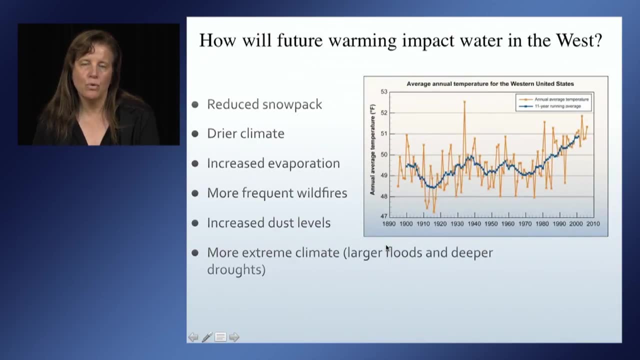 And this is when all of our water development, population growth and agricultural industry were established, And so it's possible the climate may now be shifting to a drier regime. So, in terms of future warming, how will that impact the West and California? 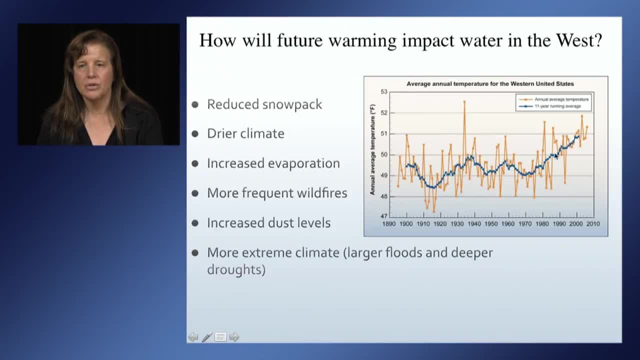 And so we're already seeing the impacts of warming. This is shown here, this warming that's been occurring since 1960.. We're seeing a reduced snowpack and that will continue into the future. a drier climate with increased evaporation rates, so drier soils. 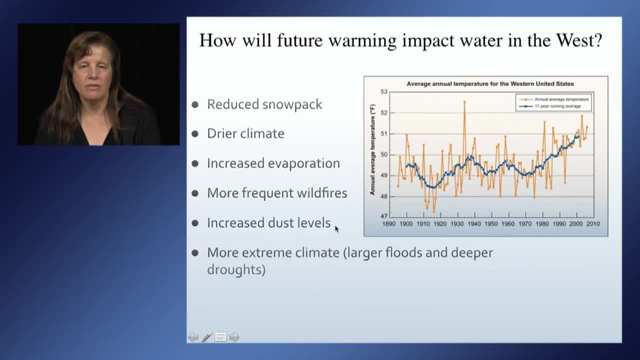 More frequent wildfires And increased dust levels as you have drier conditions and as the vegetation changes, And it's also predicted that we'll have more extreme climate. As the climate warms, you're adding more energy and more water vapor to the atmosphere.